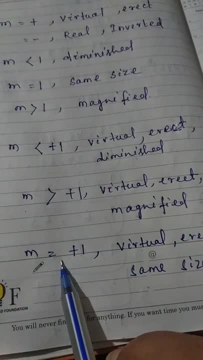 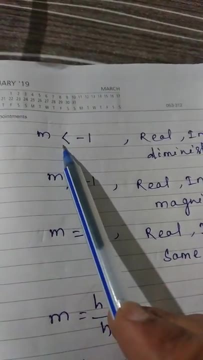 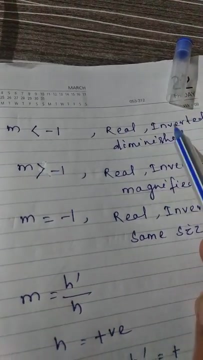 than 1 means it is magnified. Magnification is equal to plus 1 means it will be virtually erect and same size. In the same way, we can find out the magnification: is less than 1, it will be Less than minus 1, it will be real. inverted and diminished: Minus means it will be real. 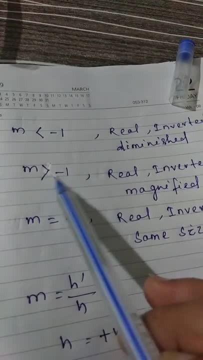 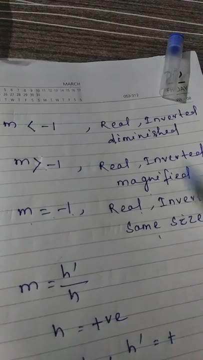 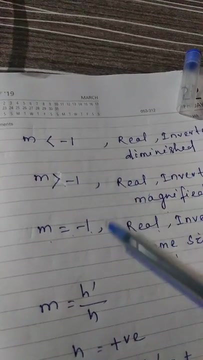 inverted and less than 1 means it will be diminished. Greater than minus 1 means real inverted, and magnified M is equal to minus 1, means it will be real inverted, same size. All these image positions you have got in your ray diagrams, Then how will find out? 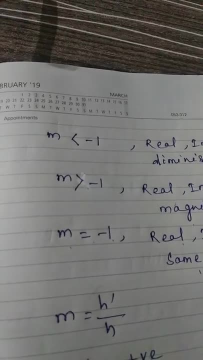 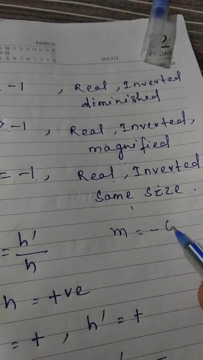 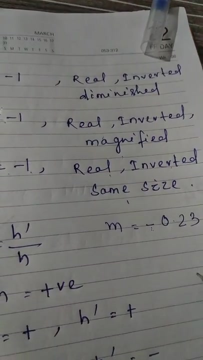 it will be If I will tell. magnification is minus 0.23.. I am giving one example. It is a magnification is minus 0.23. It is minus, So minus means it will be your real, and inverted 0.23 means it is less than 1. So it will be diminished. 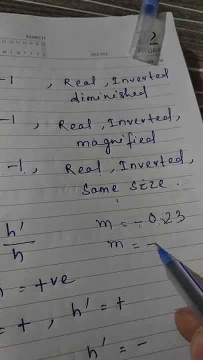 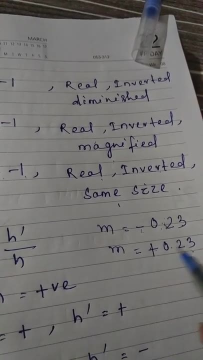 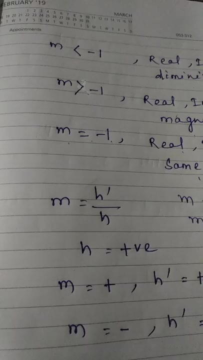 Okay, If I will tell magnification is plus 0.23, then it will be virtually erect and diminished. So here, in this way, you can find out the nature of the magnification, The image formed by the spherical mirror. Then in your mind it is coming out how it. 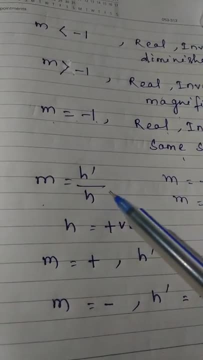 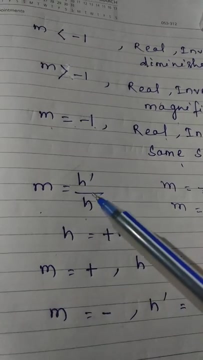 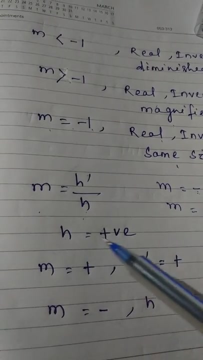 is formed how this there will be magnification formula is that h prime by h means height of the image by the height of the object. The formula is telling that how many times the image will be of the object. So always, I told you, the object is kept above the principal. 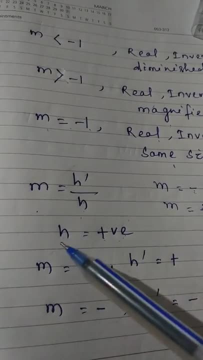 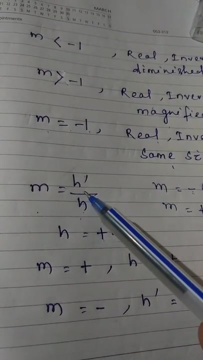 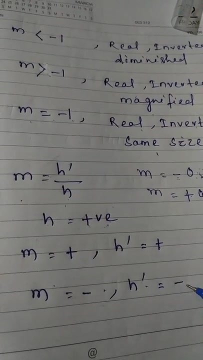 axis, So it will be positive, Means it is always positive. So if magnification is positive, means almost the image height is positive. If magnification is negative, means height of the image is negative. Height of the image is positive, means it is. 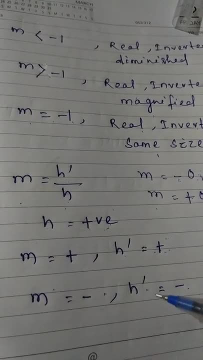 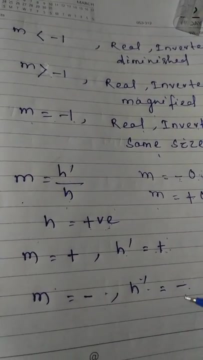 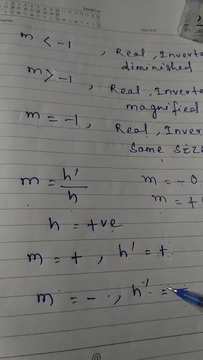 erect and it is above the principal axis And height of the image is. negative, means it is your below the principal axis and it is inverted, And inverted means it is real image. and positive Okay means. erect means it will be virtual image. Okay, Thank you.